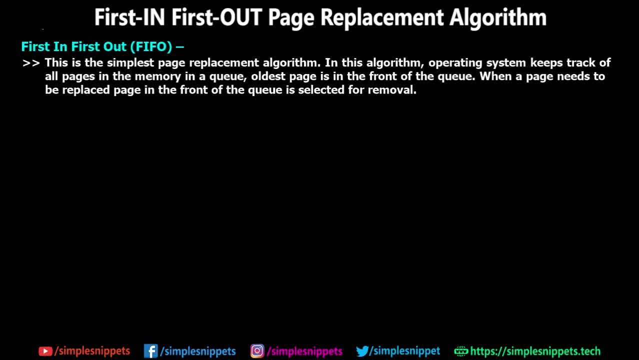 algorithm And we're also going to solve two numericals based on this algorithm. So in the previous couple of videos we've seen what is paging, what is page faults and why we need page replacement algorithms. So if you have missed those videos or if you don't, 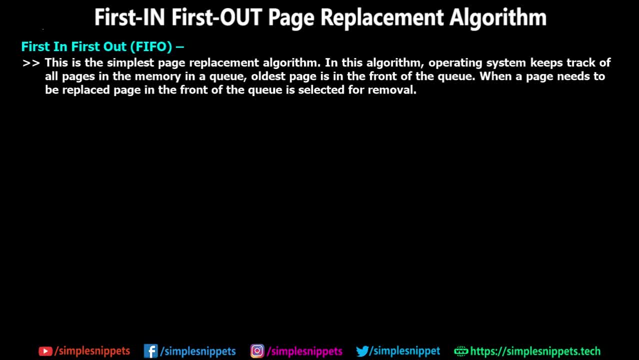 know what they are. you can check those videos in this playlist And I'm directly going to jump into the numericals without wasting a lot of time in the theory. So I'm assuming you already know what is page replacement, what is paging, what are page faults, and so 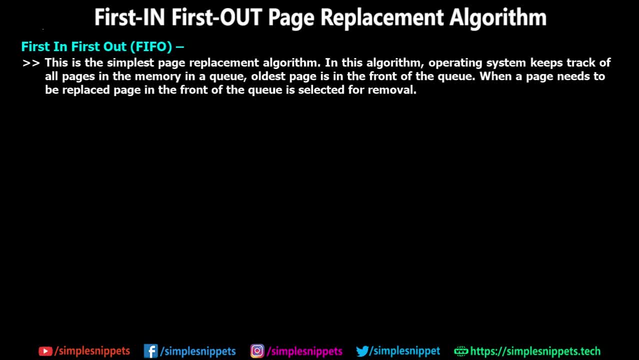 on. So, with that being said, let's start off with the first page replacement algorithm that is first in, first out. So, as the name suggests, this is the simplest page replacement algorithm that we've seen in the previous couple of videos. So let's 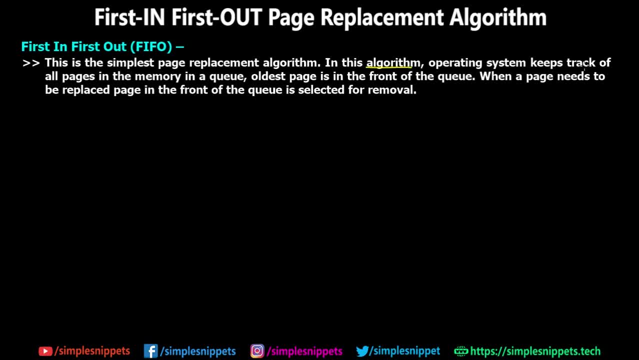 start off with the first page replacement algorithm. And in this algorithm the operating system keeps a track of all pages in the memory in a queue and the oldest page is in the front of the queue. So whenever a page needs to be replaced, the page in the front of the 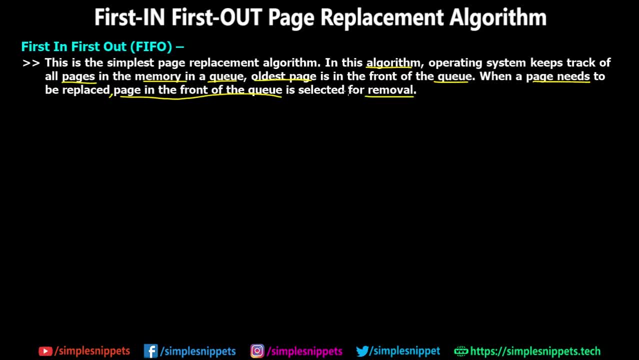 queue is selected for removal. So it is that simple. If you just read this point again, the entire walking can be imagined. but let's solve a numerical, because that is the best way to understand this. first in, first out: page replacement algorithm. So let's consider: 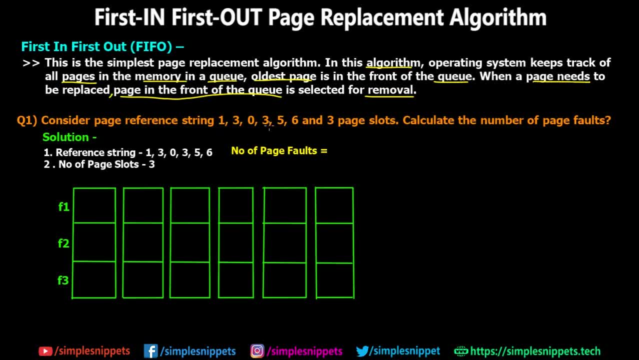 this example. So consider a page reference string: one, three, zero, three, five, six and three page slots calculate the number of page faults. So we have to find out number of page faults. We've been given a reference string and we've also been given the number of page slots that are available. 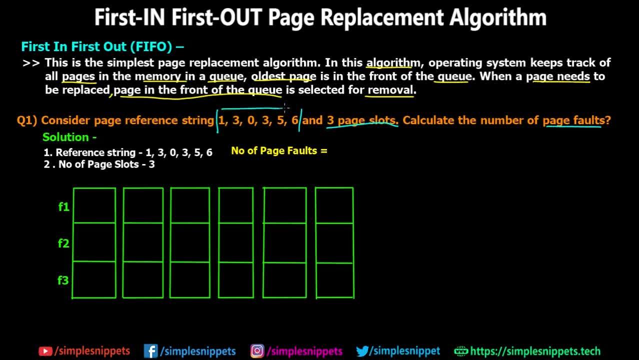 So this reference string is basically the page name that the CPU wants to execute. Okay, So the CPU wants to execute page number one first, page number three second, page number zero third, and so on and so forth. So first for simplicity, Ashley, assuming that there is only one process, let's say: 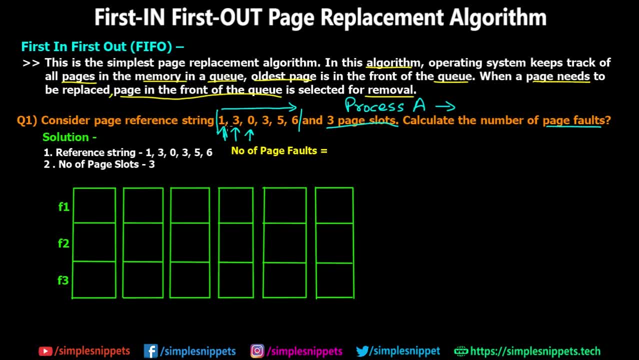 Process A and it is being divided into these: number of pages: page one, page three, page zero. So these are just names and the CPU wants to execute those pages in this order. So this is what the reference string is And the three page slots tells us that in the 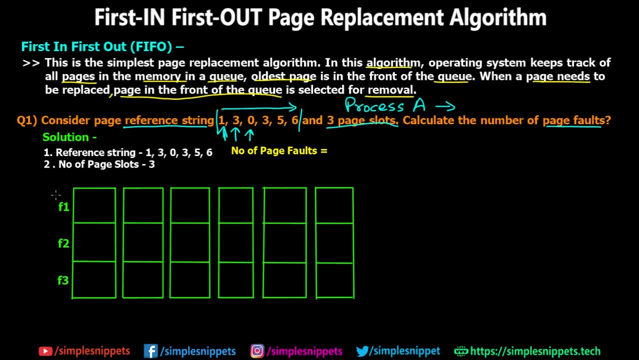 main memory. we have only three days, or three, ok. so whatever replacement I'll get them to apply. We have to apply in these three frames. so that is a content part. We have to always remember these terms. okay, Okay, and so then we'll have to create the argument. 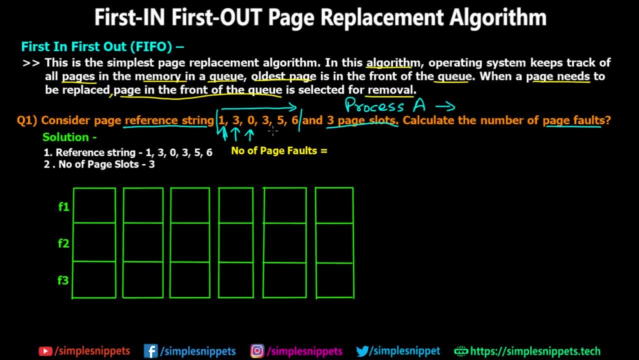 So pause, and we'll know whether or not each of them are selected somewhere under the what is depicted in this diagram. so, with that being said, let's start off with first in, first out page replacement algorithm, and you'll understand the entire working as we move through. 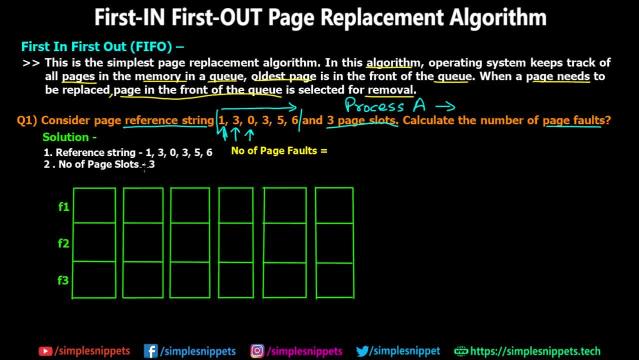 this numerical. so we have this reference string: 1, 3, 0, 3, 5, 6. so i'm just going to write it on each of this iteration. so each of this vertical column represents one iteration. so i'm just going to write 1, 3, 0, 3, 5 and 6 over here. so what do we have to calculate? we have to calculate number of page. 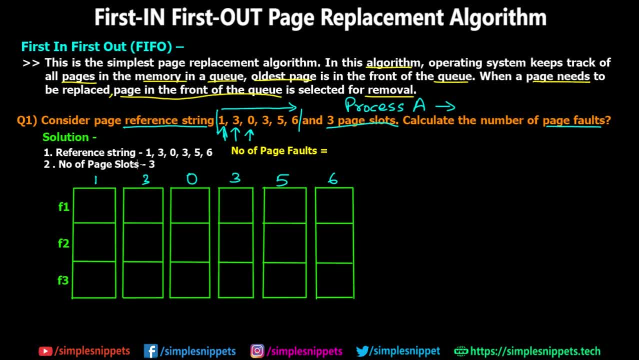 faults. so for the first iteration page 1 is requested. so you can see in the memory, in all these three frames we do not have page 1. so this means that a page fault has happened. right, so i'm just going to write x over here, or you can also denote page fault number. so this is first page. 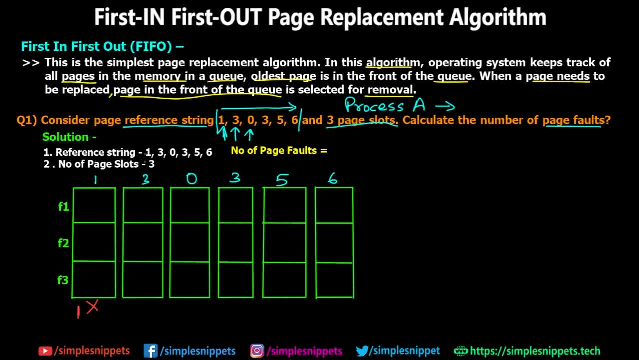 fault because it is not there in the physical memory right, which means that this page 1 has to be loaded over here. so i'm just going to write 1 over here. let's move ahead for the second iteration. cpu wants page 3. now we already have. 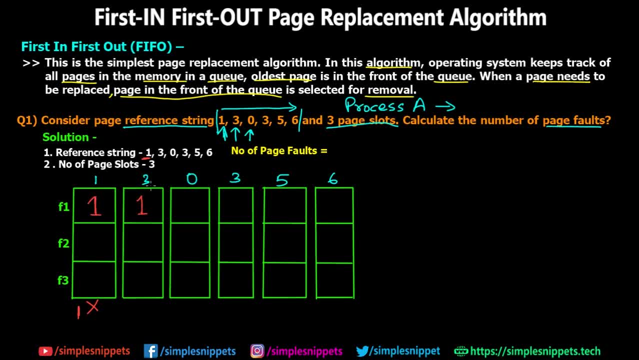 page 1 and page 2, so we have to write page 1 over here. so we have to write page 1 over here, right in frame number 1. so this is 1, but 3 is not there. so again a page fault is generated and 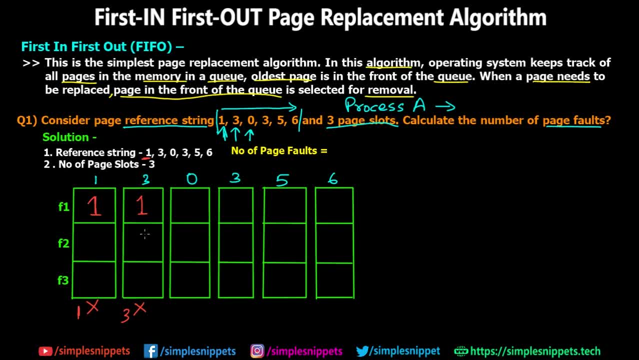 page number 3 is being loaded from the virtual memory into the main memory, so i'm just going to write 3 over here. moving on to the third iteration, we already have 1 and 3 in the memory. now cpu is wanting page 0. you can see that there is no page 0 in the frames, so i'm just going to write 0 over. 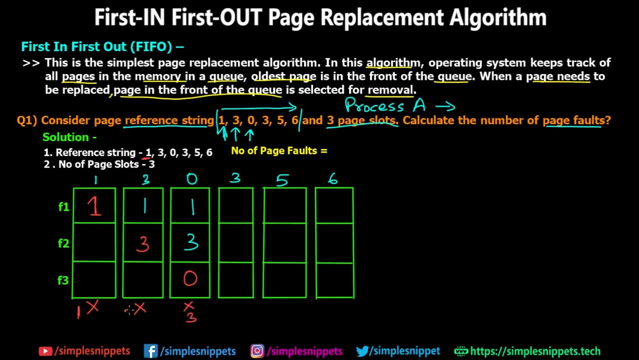 here, and this is our third page fault. this was our second page fault over here, and now for the next iteration, that is, for the fourth iteration. you can see that all the frames are filled with page number 1, page number 3 and page number 0, but cpu is wanting page 3 again, so 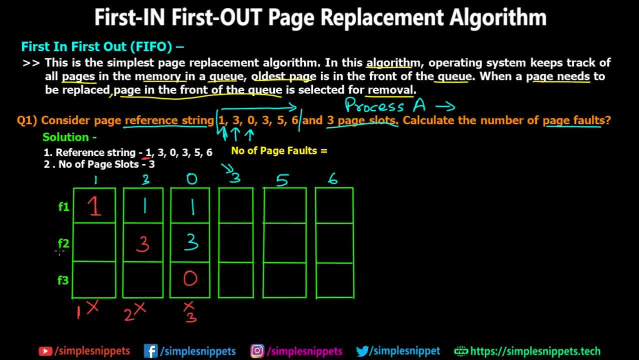 page 3 is already there in these frames right. it is there in frame number 2, which means that the page table for this process will already have an entry. that page 3 is there in the main memory, which means that page fault will not be generated. so over here page fault is not generated and i'm 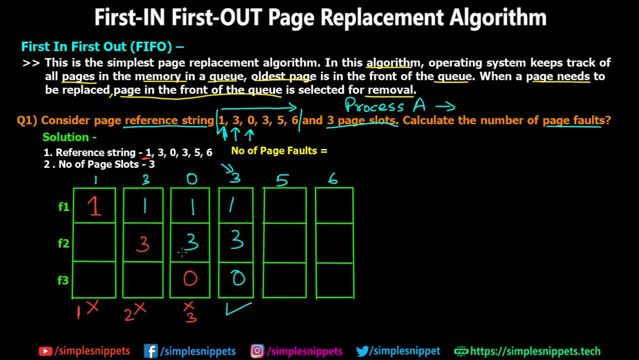 just going to write 1, 3 and 0 as it is, because 3 is already there, so i'm just going to write 1 over here in the memory. so i hope you are getting up until now. so let's move ahead now. the cpu is wanting page. 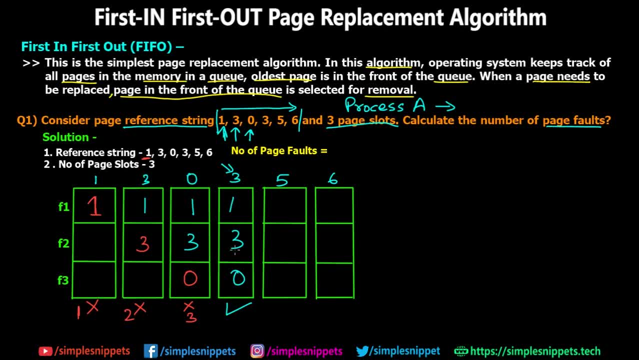 5. so you can see that page 5 is not there in these three memory slots. so we have to replace or we have to swap out one of the page, right? so this is where the first in, first out algorithm comes into picture and, as the name suggests, we have to replace the page that came in first. now, if you see from the 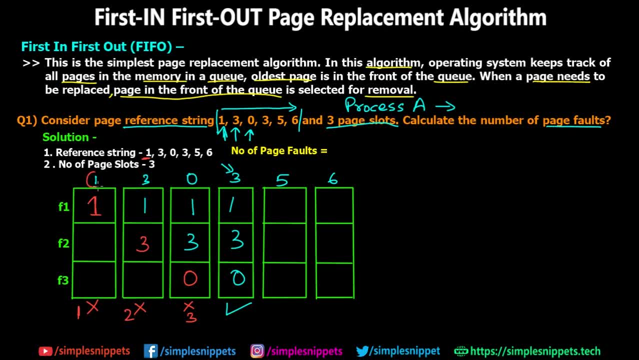 timeline. that is, if you see from the reference string order, page number one was the very first right you can see it is still there in all these frames. so that is the reason why we have to replace this one with this page five. so i'm gonna write five over here and the remaining three and zero. 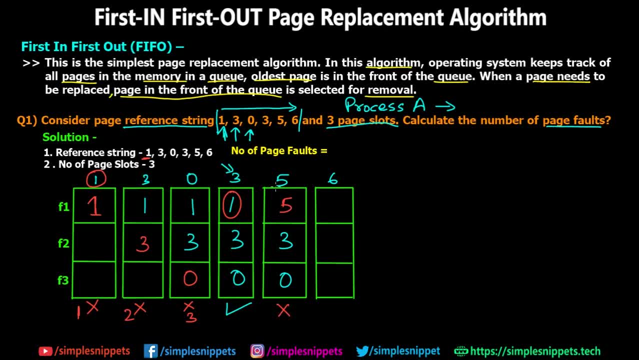 are gonna be as it is. and again, this is a page fault scenario. right, because page five was not there. it has to be swapped in in the place of one. so again, i'm just gonna mark x, and this is fourth page fault. and for the last iteration, page six is requested by the cpu. six is not there in. 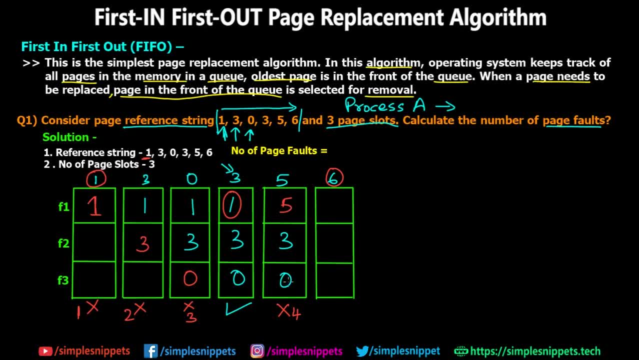 the physical memory you can see in it is not there in any of these frames. so again, a page fault is generated. so this is fifth page fault and some page has to be swapped out. so again, if you go back in this timeline or the order in which the reference string is, you can see that three. 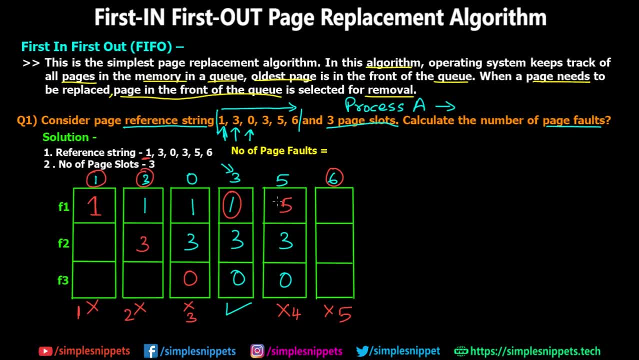 came in after one, so we've already swapped one over here in this stage. so the next page which came in right after one is three, right? so this three is going to be swapped out over here and i'm gonna write six at the place of three, and the rest are gonna be the same. so five and zero are. 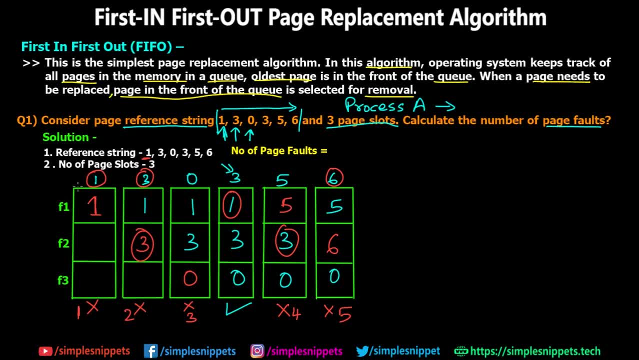 going to be the same, because three is first and second and third are going to be the same, so five in line after one, right. so that is why it is swapped out and six takes its place. so this is the entire timeline chart. you can see what is happening in the memory and the end result is: 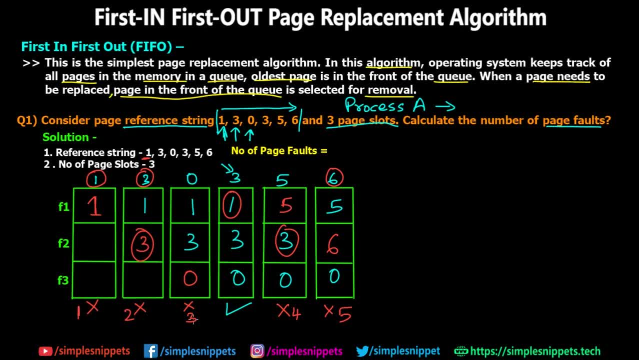 the number of page faults which you can calculate over here. so we have one, two, three. in this step page fault did not happen. we have page fault over here fourth one and fifth one. so number of page faults over here is five. so this is the final answer. so this was a very basic numerical of. 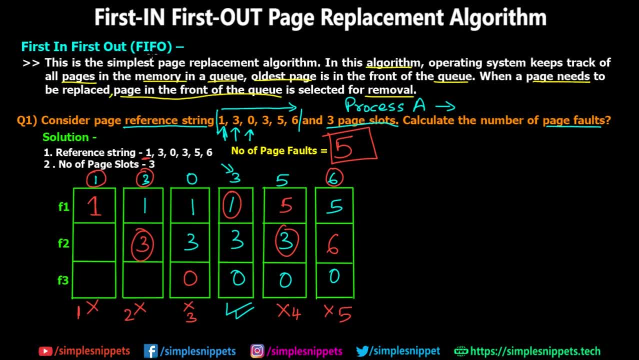 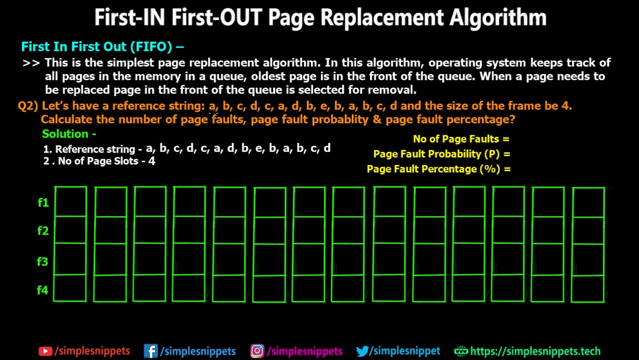 first in, first out, but i hope you have understood the overall working of how fifo works. and now let's see a little complex, rather lengthy, numerical, not complex, but a little lengthy, and there are few more details that we are supposed to be finding out in that question. okay, so in this question we have a reference string starting from a, b, c, d and. 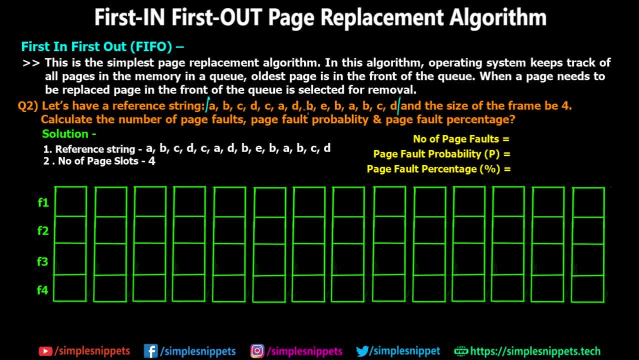 we have alphabets. so instead of numbers, we have alphabets. so basically these are page names, right? so they can be anything. and to confuse you, they can give you symbols, numbers, alphabets and so on. so it's basically one and the same thing. so we have. 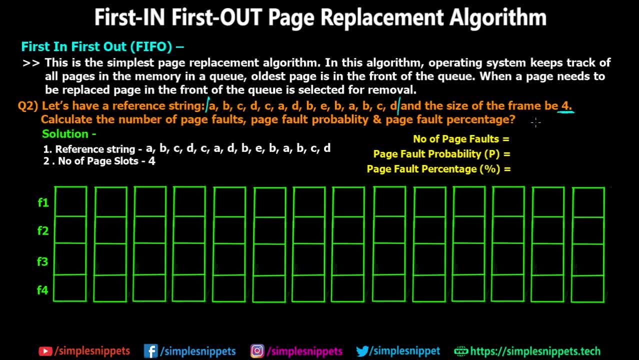 some alphabets and the size of frame is four. so we have four frames this time and not three. so the things that we are supposed to calculate is number of page faults, page fault probability and page fault percentage. so three things are supposed to be found out: one, two and three. 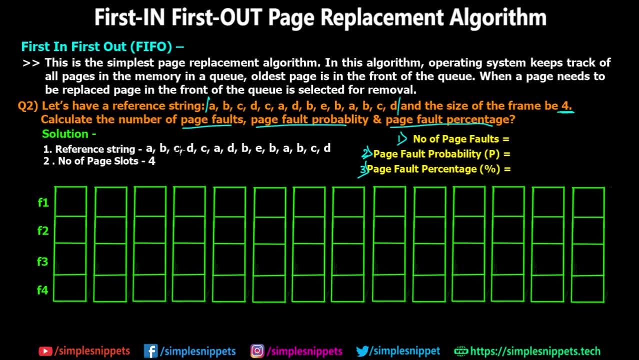 but first we have to solve this numerical, similar to what we did in question number one, just that we have four page slots, or four frames in the memory this time, and we have more number of reference string alphabets. so i'm just first gonna write down these alphabets over here. so i'm gonna 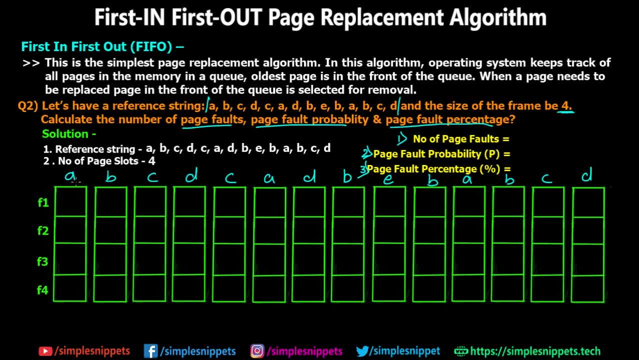 write down the alphabets. so first we have to write down the alphabets over here. so we have two alphabets here. so first we have b, b, c, d and so on and so forth. okay, so i've written down the page names in the reference string order. now let's start off with step number one. so for step number, 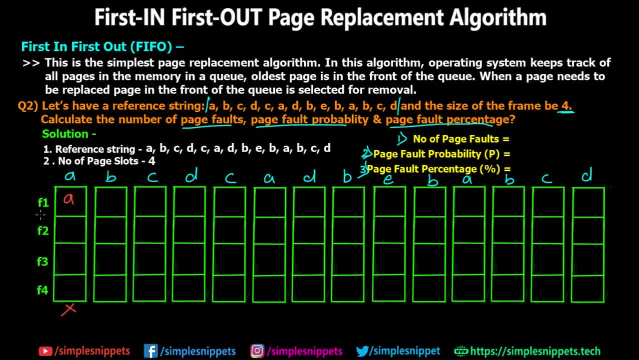 one page, a is not there in any of the frames, so a page fault is generated. i'm gonna mark x over here. i'm gonna load a in the frame f1. moving on to step number two, we have a in the memory, but we do not have b in the memory. so i'm gonna load b in the memory. and this is a page fault, because it is not. 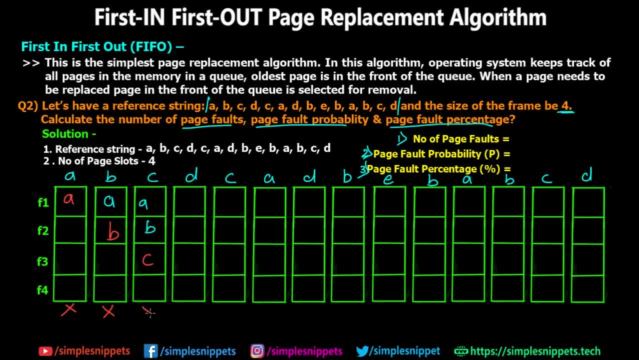 so your a and b is going to be there, c is not going to be there. so this is a page fault over here. a, b, c is there, d is not there. i'm going to load d and this is a page fault. so initial four steps. we have page faults because a, b, c, d were not there, in the memory only, which means that page. 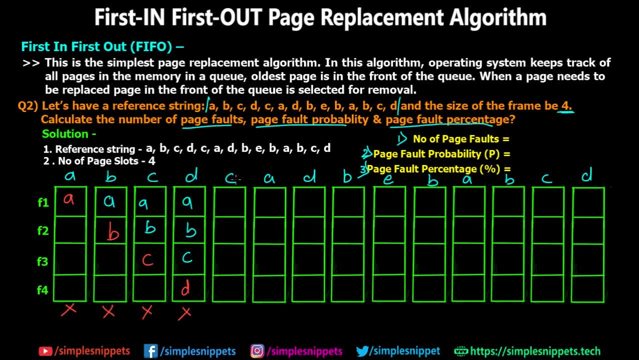 fault is happening. so for step number five you can see that page c is already there over here. so page fault is not going to happen. so i'm just going to write a, b, c, d as it is again, similarly for a and d. that is step number six and seven. same case right. so a, b, c, d again here. a, b, c, d. so 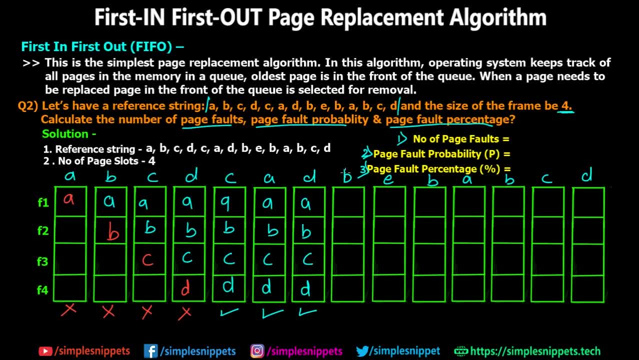 no page fault here and here, similarly, for this step, that is requesting b. so b is already there in memory. so again, no page fault writing a, b, c, d as it is. but now at this step, the cpu is wanting page e. up until now we never had page e in the memory. we have only a, b, c, d, so one of the page. 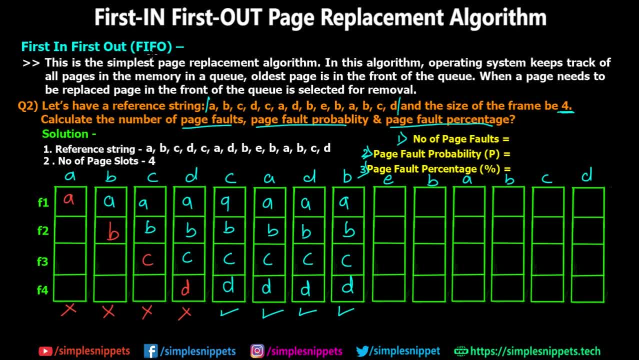 has to be swapped. now, according to fifo, first page that came in has to be swapped and if you see, if you go back in the timeline, you can see a came in first and it is still there throughout all these steps, which means that a has to be. 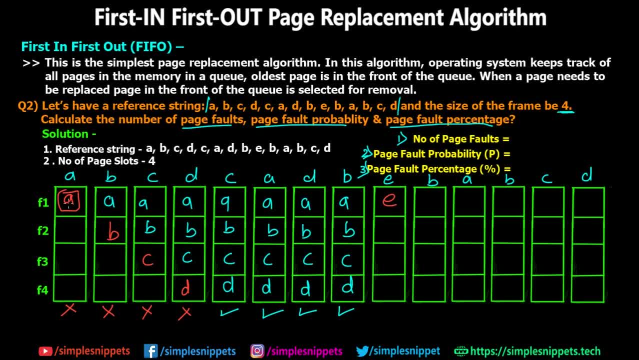 swapped out, right, so i'm going to write e at the place of a, that is in frame one, and rest of the things are going to be as it is. so b, c, d are going to be as it is, and this is a page fault situation, right, because we had to perform swapping, which means e was not there in the memory, so it had to. 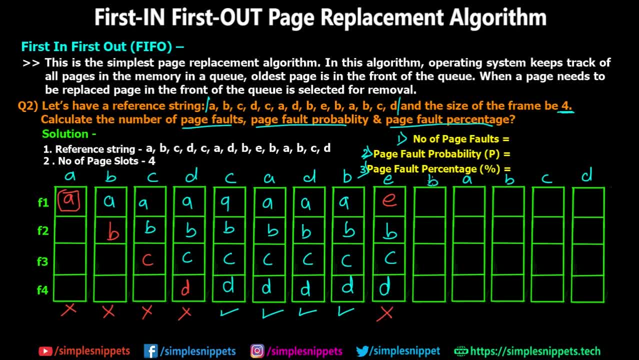 be swapped out. so right now, having this gone fails the next step. we want that. we want a memory start over here, so we need to swap everything in memory. you can see here that you're going to get b, so you need to write my relatively free memory. this is a page fault. 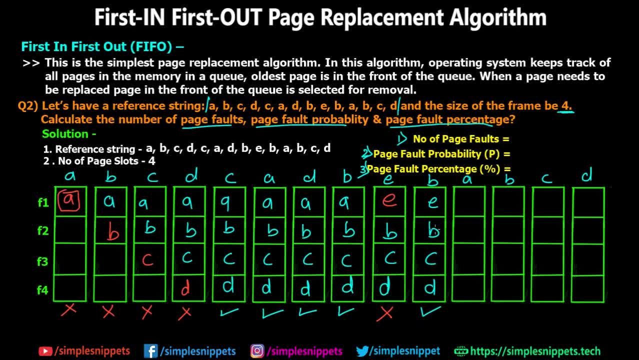 situation. i'm just gonna mark x. let's move to the next step. we want b over here. b is already there in the memory, so i'm just gonna write everything as it is: e, b, c, d. this is not a page fault. moving on to the next step, we want a in the memory, but a now is. 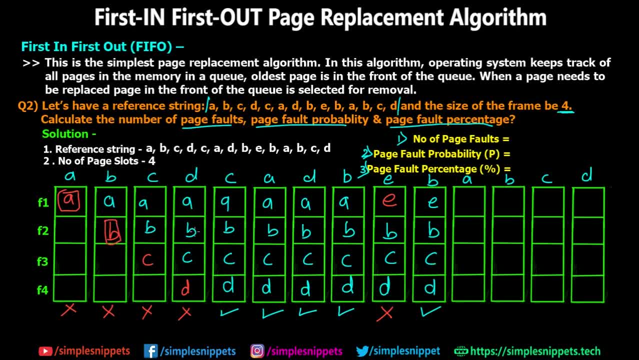 not there in the memory because we swapped e instead of a right, so a has to be brought in the these steps, so b has to be swapped out for the next iteration and a is going to be loaded in place of b and rest. things are going to be as it is, so ecd is going to be as it is and this is a. 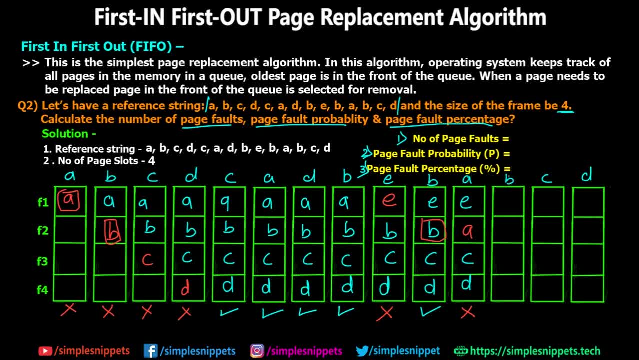 page fault scenario. now moving ahead for the next step. b is requested, but in the previous step we just replaced b, right? so we have to again bring back b from the virtual memory into our physical memory. so which page should we replace? so, according to fifo, after a and after b, c was brought into the. 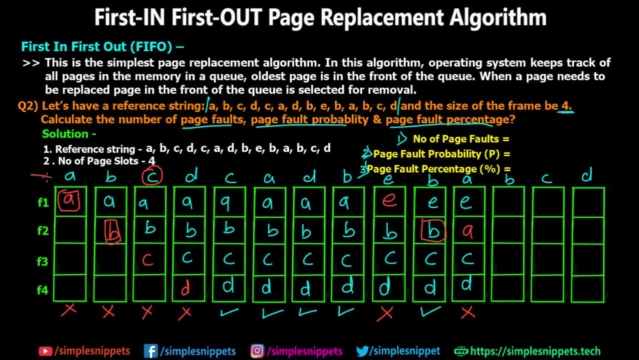 frames right. you can see in the timeline that is in this order. so c is still there. you can see c is there throughout all these steps. so now we have to replace c and instead of c we have to add b, and rest of them are going to be as it is. so e is going to be as it is, a is going to be as it is, and 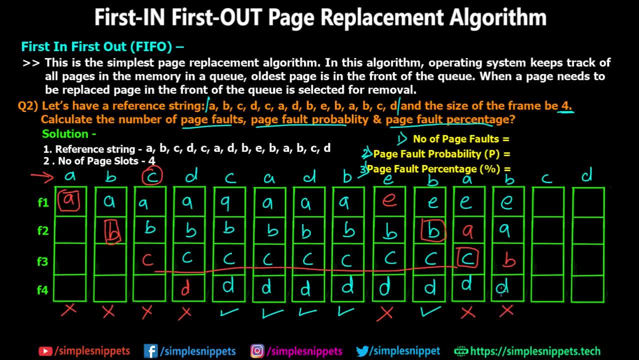 d is going to be as it is and this is again a page fault scenario. moving on to the second last step, cpu wants c, but we just replaced c in the previous step, so c has to be again brought back in the memory and if you observe in this entire timeline, d was brought last and it is still there, so it came in first. 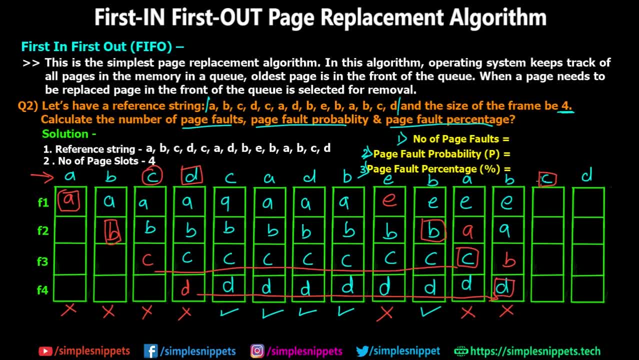 right compared to others, so we have to swap out d now. so instead of d we are going to add c. over here it's a page fault and rest of the things are going to be as it is. so i hope you are understanding why we are replacing page number b, c and d in all these steps, because they were the first which came. 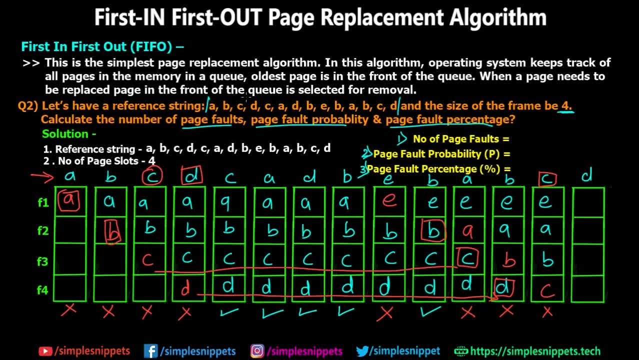 in and that is why they are going to be the first which are going to go out, because, according to history, they came in 2 and they need one page paste. there is no page työ, it is just there to match their size. so d has to be replaced, right? ok, so now we are on the last step. 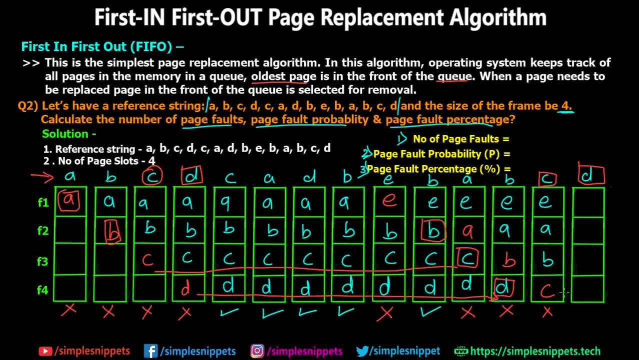 and now we want d, but d is not there in this four frame. so again a page fault is generated and now we have to swap one page out of these 4 pages. so which one should we swap? so if you observe, in this step c came in, in this step b came in, in this step a came in, and in this step b came. 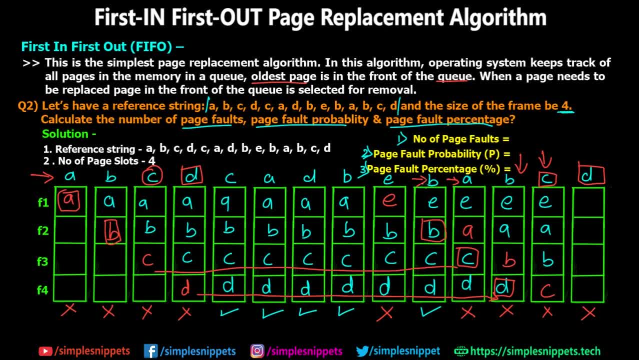 in. so we cannot replace c, we cannot replace b, we cannot replace a and we cannot replace b again that this e is the oldest page compared to a, b and c. so a, b and c came in recently, but e is the oldest page, which means that it is first compared to a, b, c. so we have to replace e now and instead. 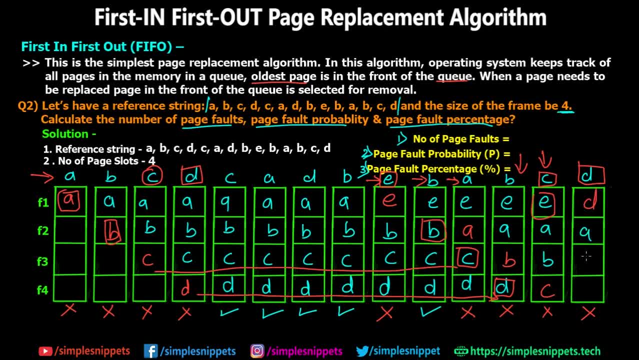 of e, we have to add d and the rest of them are going to be as it is. so a, b and c are going to be as it is, and this is a page fault situation. so this is the entire numerical and we still have to calculate these three values. but i hope you've understood how to go about this reference string. 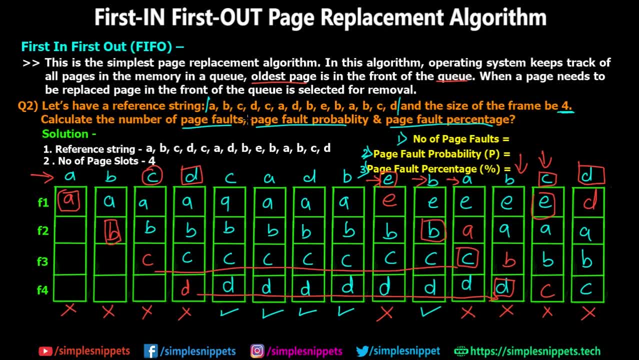 and memory allocation and swapping of pages using first in, first out page replacement algorithm. now let's calculate these three values, so the number of page faults you can easily calculate. so this is one, this is two, this is three, this is four, five, six, seven, eight and nine. so number of page faults: 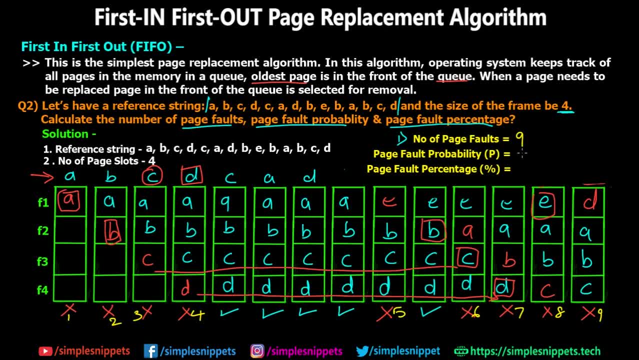 is nine. now the page fault probability is given by number of page faults. that is, nine divided by the total number of memory accesses, which is fourteen in this case. so if you just count the alphabets in this reference string, so we have one, two, three, four and so on and so forth. it is: 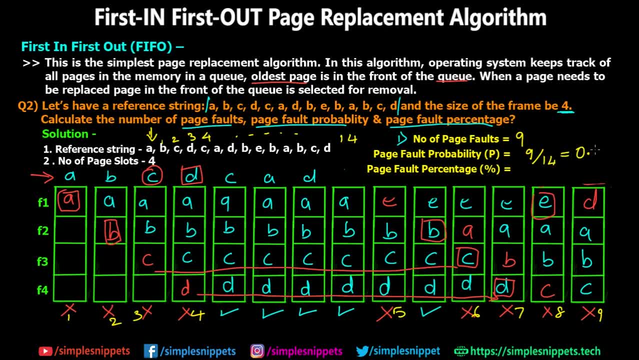 fourteen. so nine by fourteen is gonna give you zero point six four two. okay, so this is the page fault probability, which means that the probability of a page fault happening in this system, in with this reference string and with this first in, first out algorithm, is zero point six four. so, lastly, the 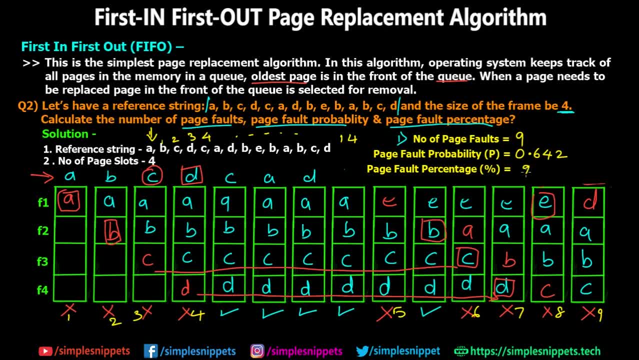 page fault percentage is number of page faults, which is nine, divided by the total number of memory accesses, which is fourteen, and into hundred. so this is basic percentage formula. in fact, if you just multiply 0.64 to into 100, you'll get 64.2 percent. so this is the final answer. okay, so yeah. 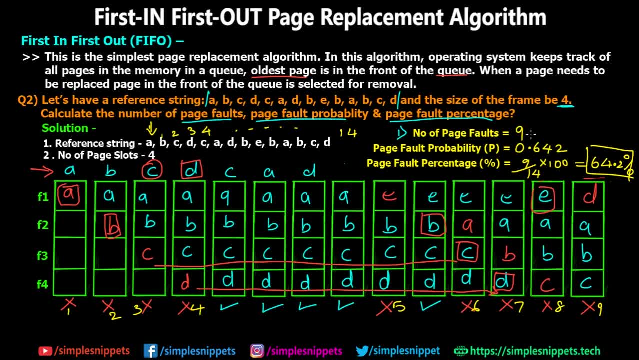 this was the first in first out page replacement algorithm and we saw the theory, what is first in, first out, and we also solved two different numericals. first one was pretty easy, wherein we understood how fifo works, and second one was a bit lengthy but definitely not difficult, and we had 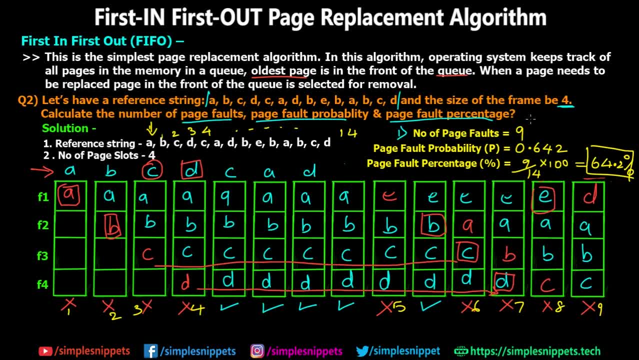 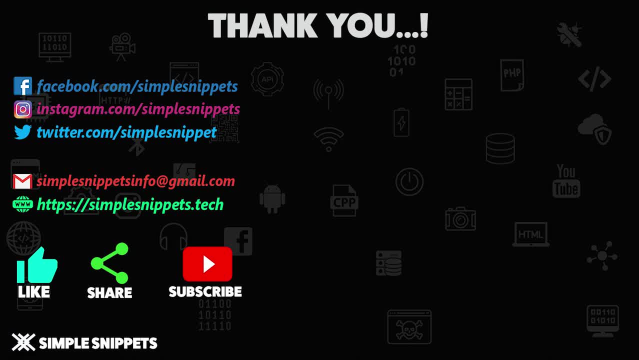 three different values in this case, so i hope you have understood the entire numerical and that's it for this video. guys, i hope you like this video. if you liked it, please give it a thumbs up, share it with your friends, comment and let me know how this video was. if you haven't yet subscribed on: